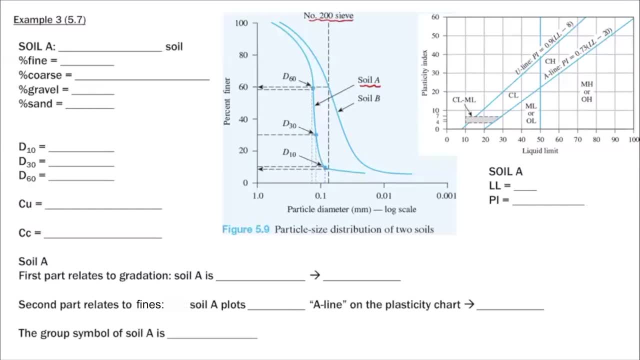 So the number 200 sieve corresponds to a particle size of 0.075.. That's a threshold value separating coarse-grained soil from fine-grained soil And if you look at this figure here for soil, A curve, this percent passing, which is the y-axis, that's a little bit less than 10%. 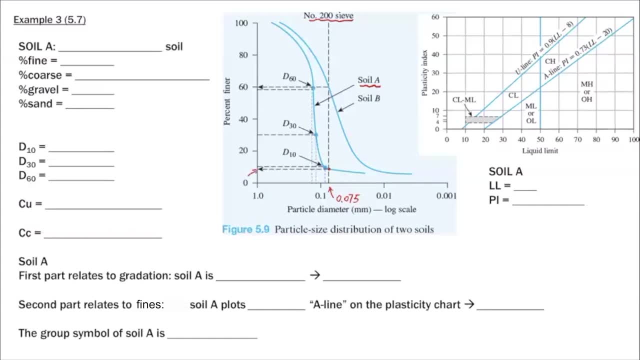 This value here, that's a percent passing number 200 sieve. It's about 8%. You can read this directly from the curve. So this means that 8% of the soil is finer than 0.075.. We're number 200 sieve, So that's the percent of fine. 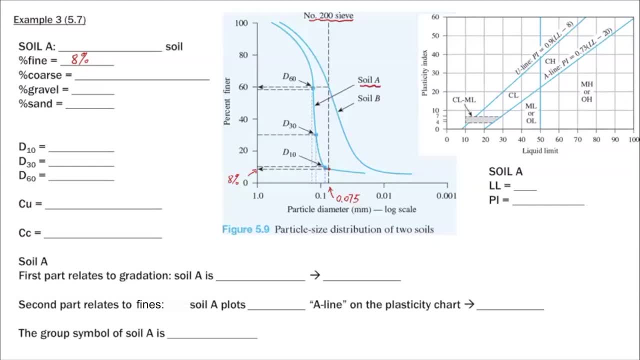 And then the percent of coarse is 100 minus that. So it's 100 minus 8% And we can tell soil A is a coarse-grained soil because you have more coarse-grained coarse than fines. So that's coarse And we know we're going to use the upper portion of that table. 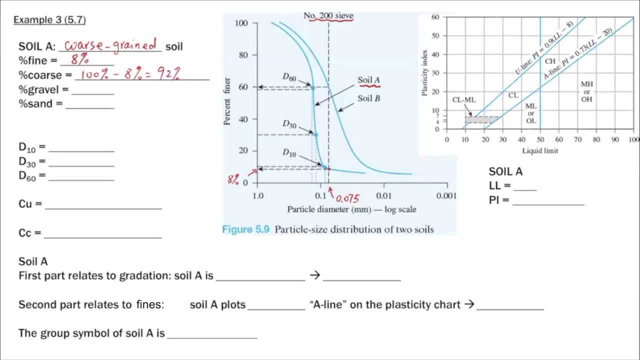 5.2, that's our classification table. That's, of course, grain soil And then percent of gravel, and percent of gravel is basically the percent of soil larger than 4.75mm. And if you look at this particle size distribution curve, you notice that 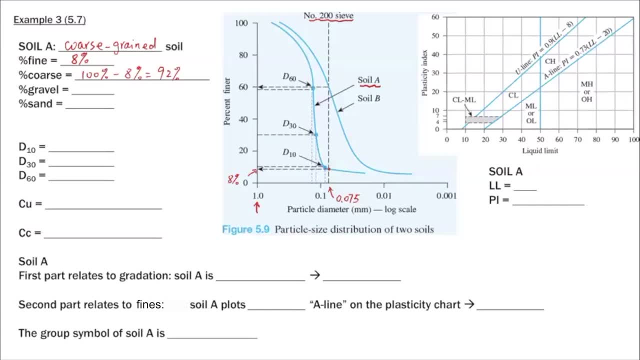 the largest particle is 1.0.. So 100% of soil passes is 1.0mm, which means 100% of them will pass 4.75.. 4.75.. the percent of gravel is 0%. Again, how we get this is because all soil 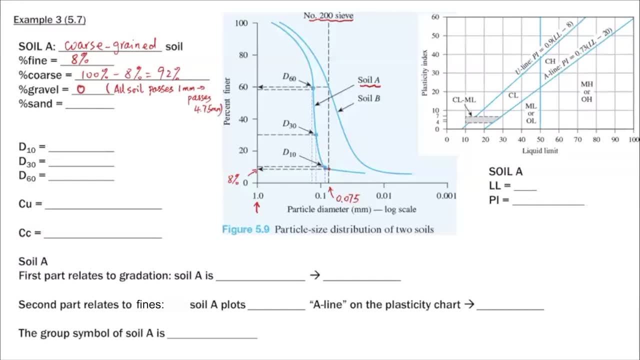 from that PSD curve. we know 100% of the soil passes at one millimeter. so that's your largest particle size, which means 100% will pass 4.7 millimeter. So gravel percent is zero, And then percent of sand is, in this case, 92%. 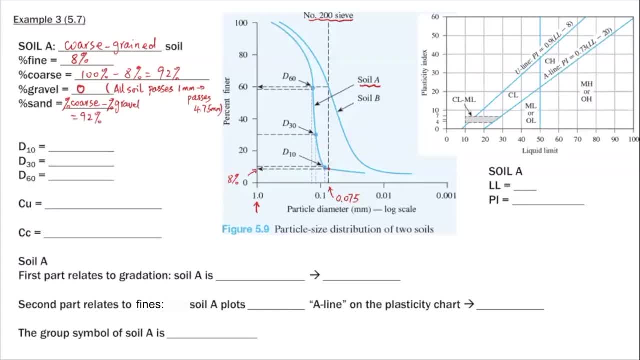 So that's the percent of different types of particles in this soil sample for soil A And also from this PSD curve. since it's a coarse-grained soil, we'll need these D values and these two coefficients. So D10 definition is the particle size. 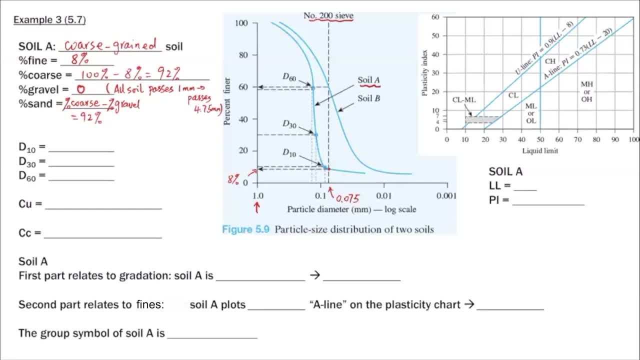 corresponding to 10% of final. So I'm going to start from 10% and then find the corresponding particle size which by definition, is D10.. So this value here, This D10.. Again, something you read directly from this curve. 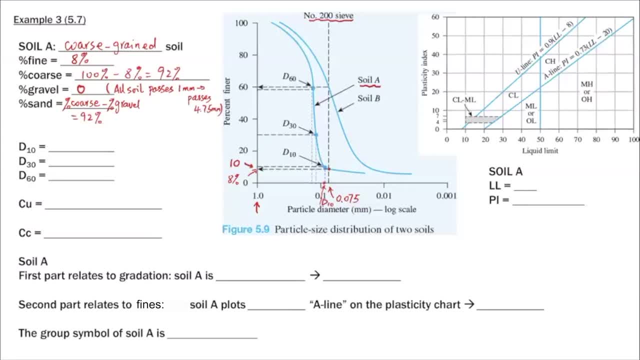 from this X axis it's about, it's a little bit smaller than 0.1.. So about 0.085 millimeter And D30, by definition particle size corresponding to 30% final. So we start from 30% on the Y axis, so 30% final. 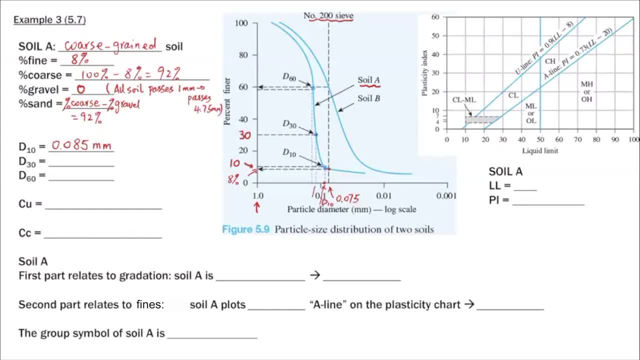 Then the corresponding particle size by definition is D30.. It's a little crowded here, So that's a D30 value. You read this from this X axis about 0.12.. And then last the D60.. Again, start from 60% of final. 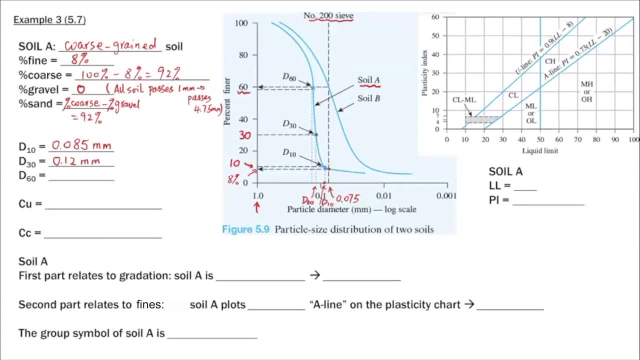 find the corresponding X axis, the particle size, So this part here that's D60. And this is about 0.13.. And this is about 0.135.. Once you've got these D values, then Cu and Cc, these two coefficients. 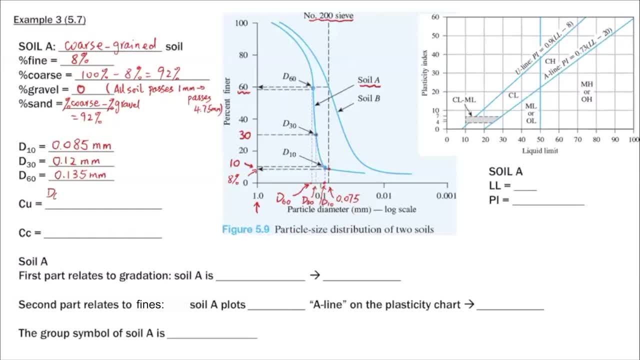 you can calculate their values using their definitions. These are the values of Cu and Cc: 1.59, 1.25.. And the last piece of information we have for soil A is the adiabatic limit test results. So we have the liquid limit for soil A: 30. 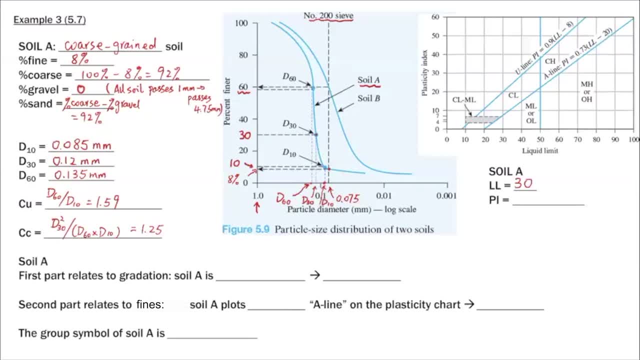 And then the plastic index is LL minus PL, And PL is given, which is 22.. So LL or PI is eight. So that's all the information we have for soil A, And then let's use that table 5.2. 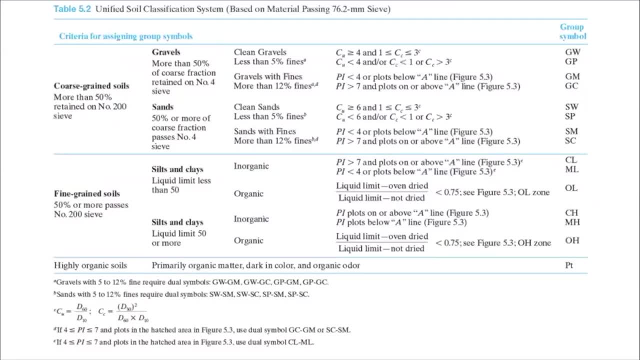 to find the group symbol first. So this is table 5.2.. As I mentioned, we're going to use the information we just obtained for soil A to guide us through this table. So enter from the left-hand side And the first decision to make is percent of coarse and fine. 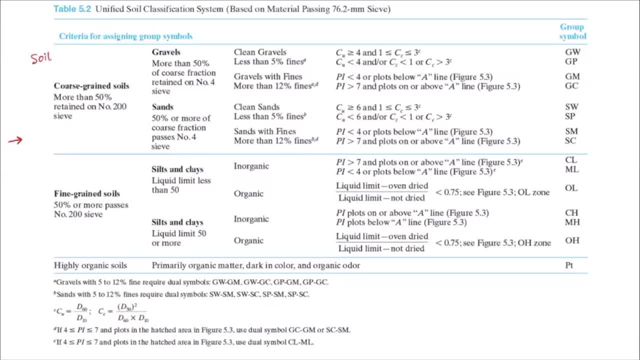 So if you look at the percent of coarse and fine for soil A, so based on this, we know this is a coarse grain soil. So the first decision is to pick that upper portion of the table And then we're going to navigate through this table using 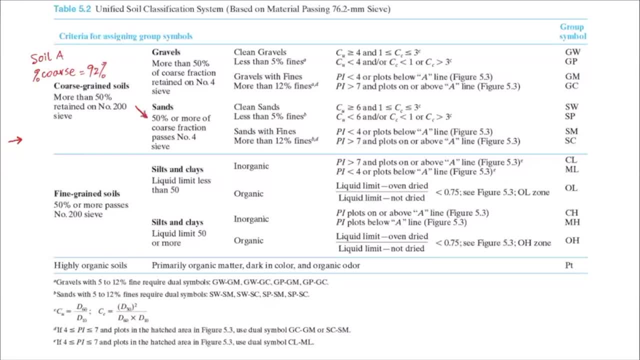 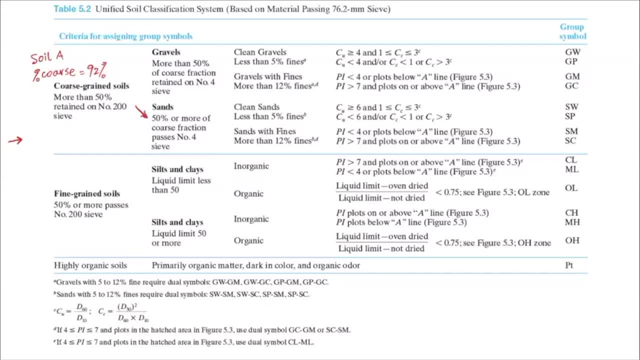 So we have more sand than gravel. So this statement here- 50% or more of coarse fraction- passes number four, sieve. In other words, this basically means you have more sand than gravel For our soil. remember: 92% versus 0%. 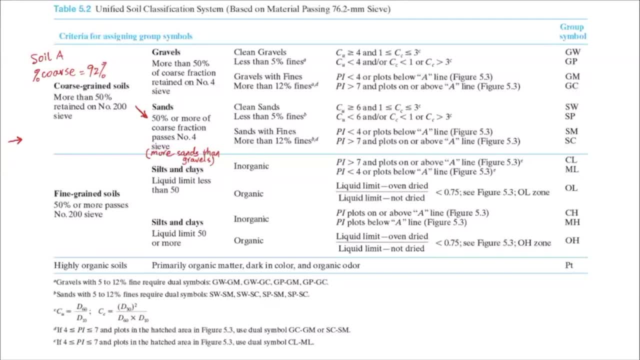 So we have more sand than gravel. So we go this route here. And then the next. this criteria is based on the percent of fines For soil: A percent of fine. And then the next. this criteria is based on the percent of fines. 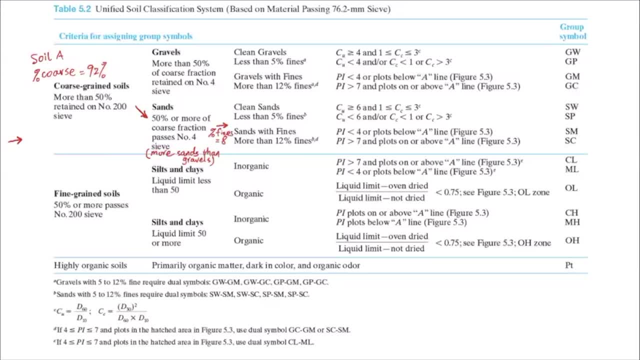 For soil B, percent of fines is 8%. And this 8% if you look at both criteria here, one is less than 5,, one is more than 12.. So this 8 actually sits in between, And that's where that footnote comes into play. 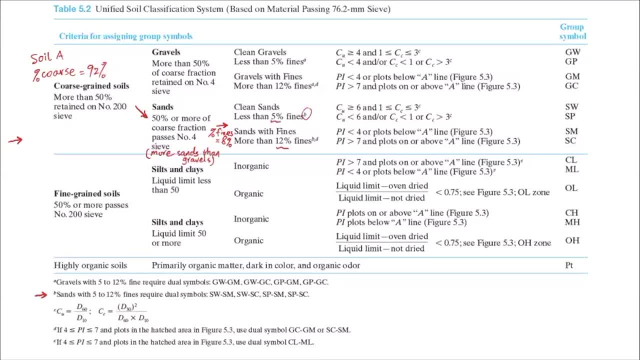 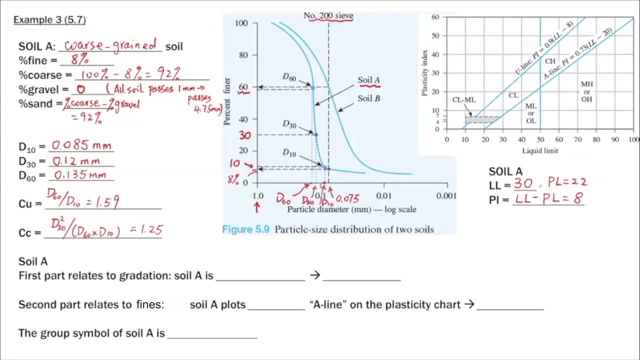 So if you look at footnote B, sand with 5% to 12% fines require dual symbols. We have 8% of fines, So we're going to use dual symbol And to find dual symbol. so for dual symbol of coarse grain soil. the first part relates to gradation. 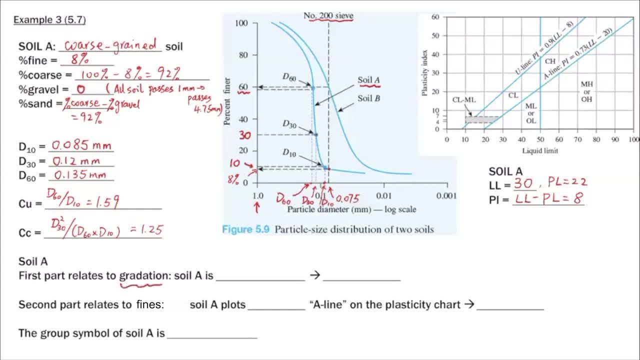 So first let's look at this soil A. So we know it's a sandy soil. We have more sand than coarse, So we need to determine its gradation. So we have these two coefficients, Cu and Cc. So right here for sandy soil, for soil. 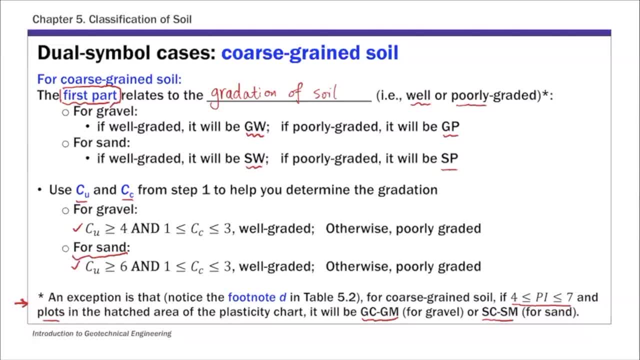 to be categorized as well graded, you have to meet both criteria: Cu greater than 6. And Cc between 1 and 3. If you don't meet either one of them, the soil is classified as poorly graded. So let's go back to our example. 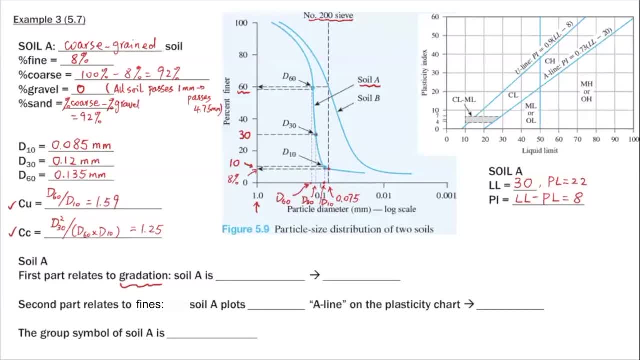 In our example, the Cu value for soil A is 1.59.. So this is smaller than 6. So it doesn't meet both criteria for well graded. So this soil A is classified as poorly graded soil And, as I mentioned, this is sandy soil. 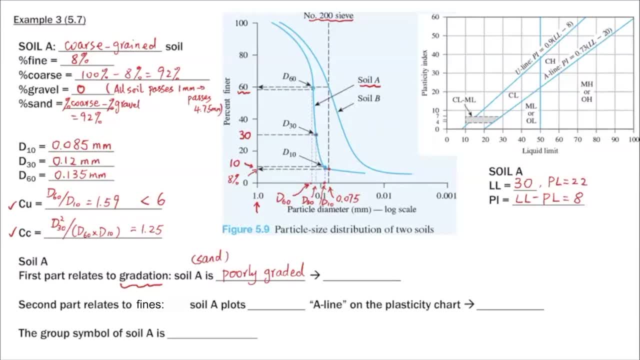 So we have more sand than gravel. So this, the first part of the dual symbol, is therefore Sp, S for sand, P for poorly graded. So that's the first part of the dual symbol. So the second part relates to fine contents. 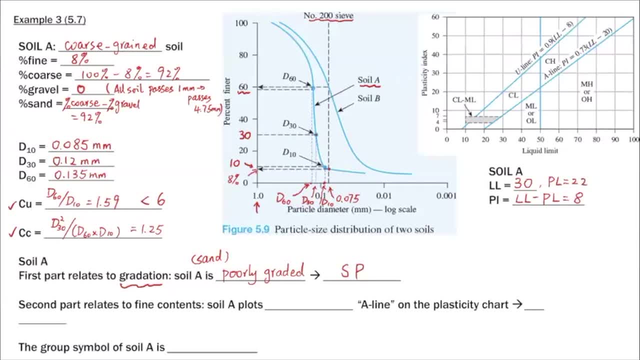 And for soil A, to determine the fine contents we just use the Plasticity Chart and that A line. So soil A, LL of 30,, Pi of 8, plots right here. Soil A plots just above the A line, So the fine contents are actually clays. 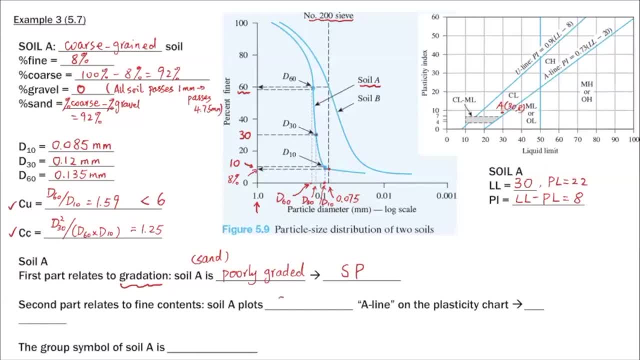 We know the second part of the dual symbol. In this case this is Sc, S for sand, C for clay. So that's the fine contents in soil A is clay. So the group symbol of soil A is, you combine these two, Sp, Sc. 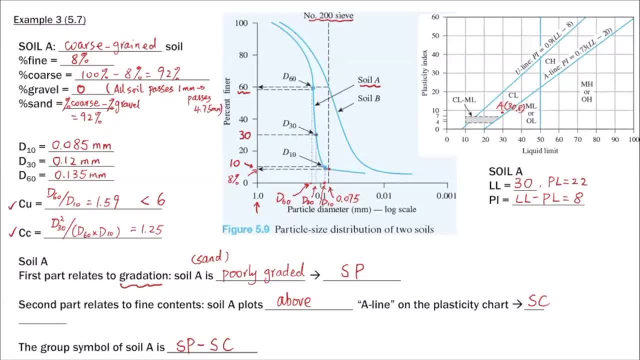 And then one thing I want to point out here. So if you're a point like this example plots very close to A line, so how can you tell if it's above or below A line? So a quicker way to check, let's say for LL of 30.. 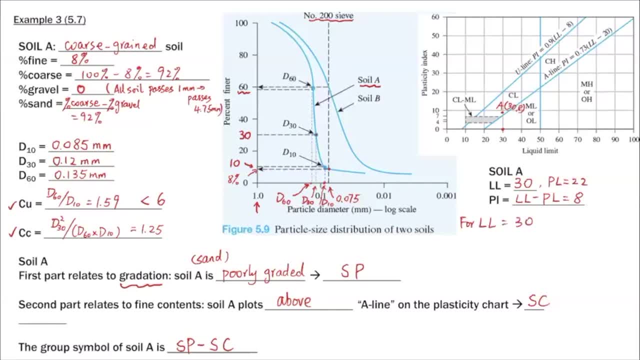 The Pi value on the A line can be calculated using the A line equation. So you can actually pinpoint that Pi value on A line. So on A line, So you can actually plug in your PI value from that A line. So you can actually plug in your PI value on A line. 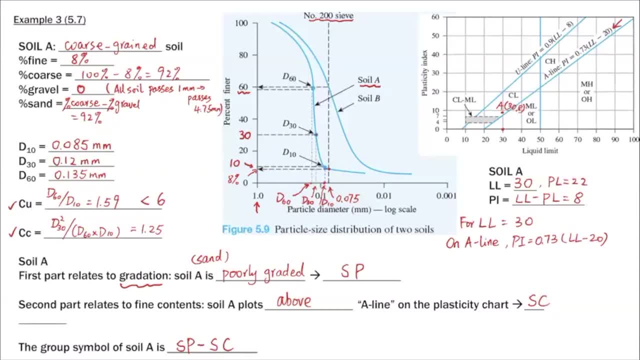 liquid limit to see where that PI on A-line is. For this soil this is 7.3.. And the plus index of your soil is 8, so it's a larger, greater than that PI value on A-line, so it's actually above A-line. So this is when the two points are very 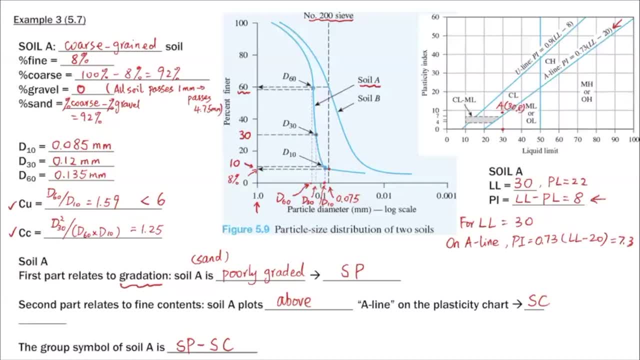 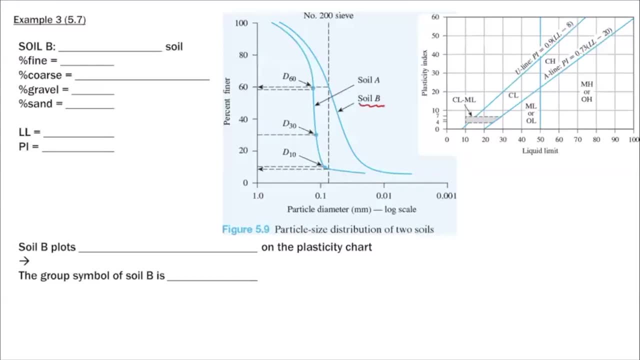 close. You can use the A-line equation to basically pinpoint where that A-line value is. So for soil B, we're going to focus on this curve here And the percent finer corresponding to number 200, Steve. so remember that's 0.075 millimeter. So 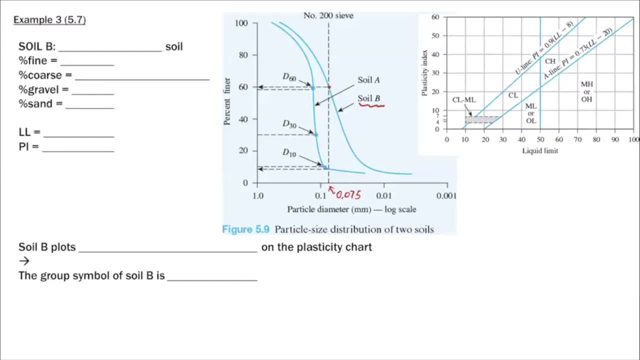 the percent finer for this soil B is, if you read this value from the curve, about 60%. So that's the percent finer. And then the percent coarse: 100% minus that And percent gravel, just as previous example, previous soil A: 0% And then sand is 40%. 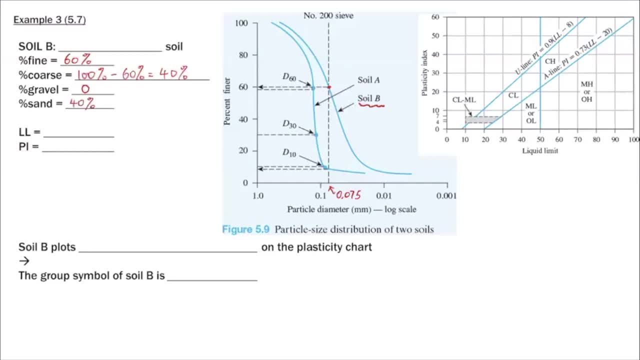 So soil B is a fine-grained soil, So you have more fines than coarse, so that's a fine-grained soil. And LL value for soil B is 26. And PL is given it's 20.. So that's all the information given for soil B And this is a fine-grained soil. 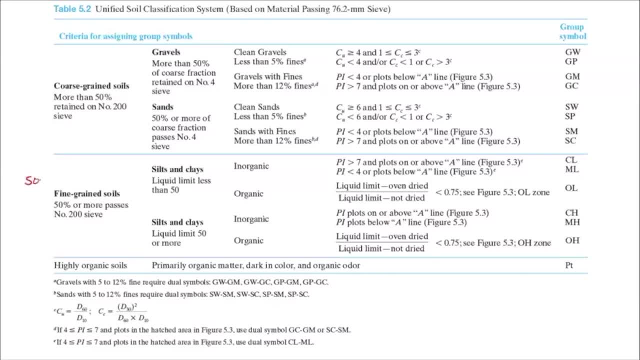 We're going to use this bottom portion of this table And the liquid limit of soil B 26,, so that's less than 50. And for this soil, unless it's otherwise stated, all the soils we're going to deal with in this. 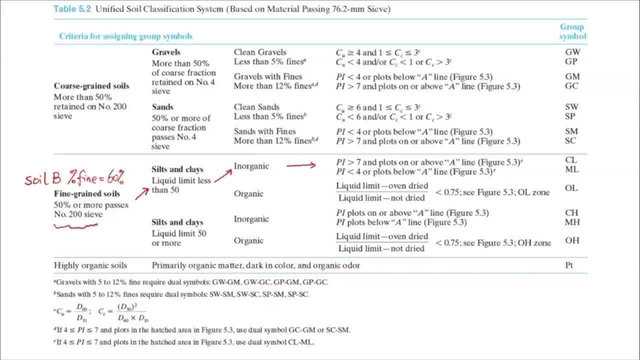 course are inorganic soil, And then the PI value for soil B is 6.. So that's in between 4 and 7.. So we need to pay attention to this footnote E here, And footnote E is for a soil that has PI value between 4 and 7. n plots in the hatched area. 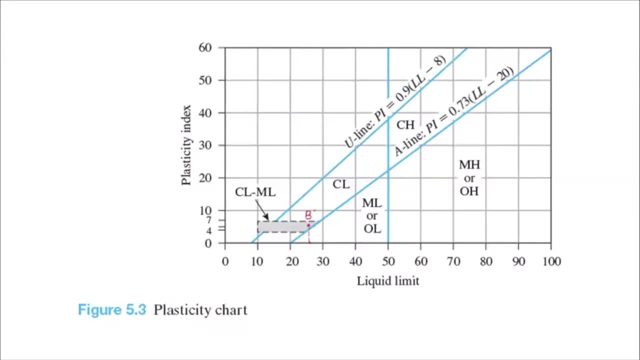 So that's the due symbol Cl-ML. So let's check that. LL values 26.. So this is soil B. So this soil B is 26ужеkur and six, so it plots in the hatched area. 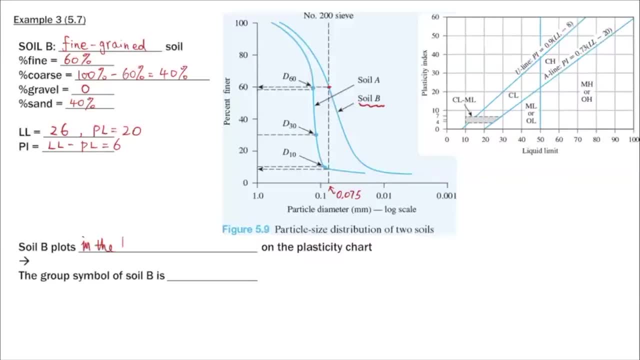 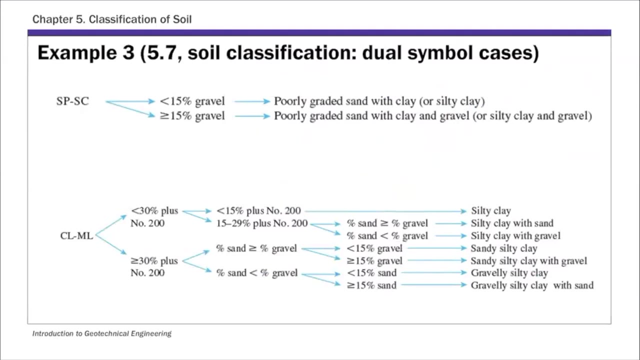 So the symbol for soil B is CL and ML. Okay, so that's the group symbol for soil B. Again, a dual symbol case. And finally, once we have the group symbol, the next information we need is the group name. So, for soil A, 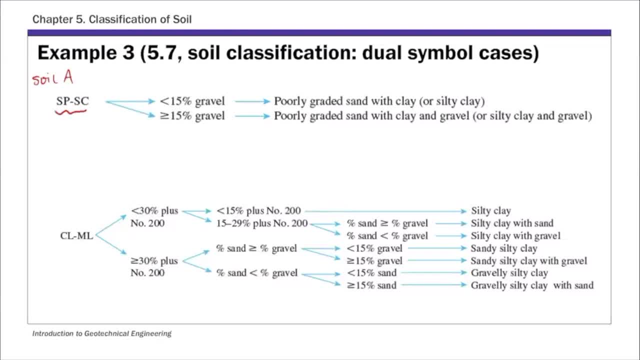 So we start from the group symbol we just found and then just navigate through this table, this figure, to find the group name. So we have 0% gravel for soil A, so that's less than 15.. The group name of soil A: